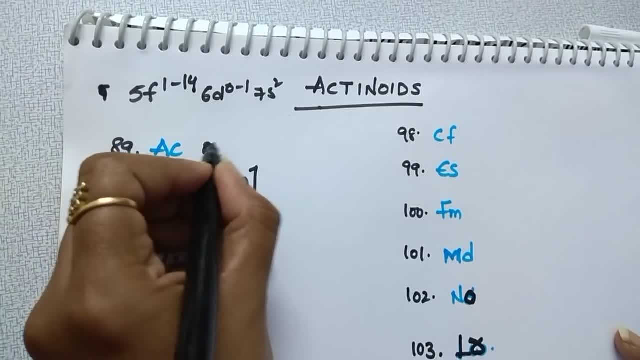 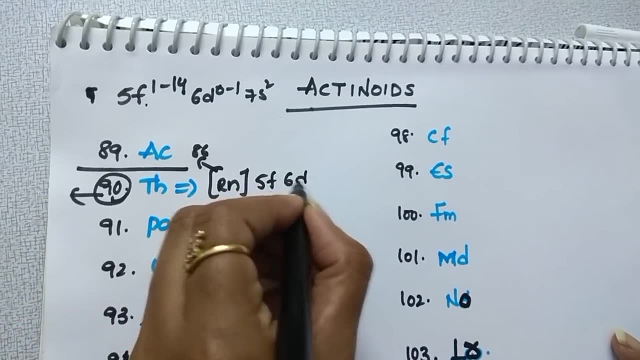 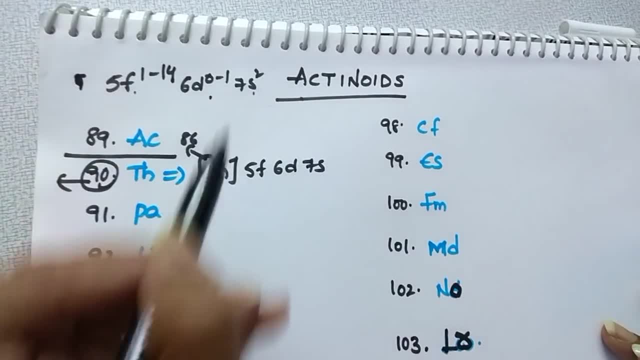 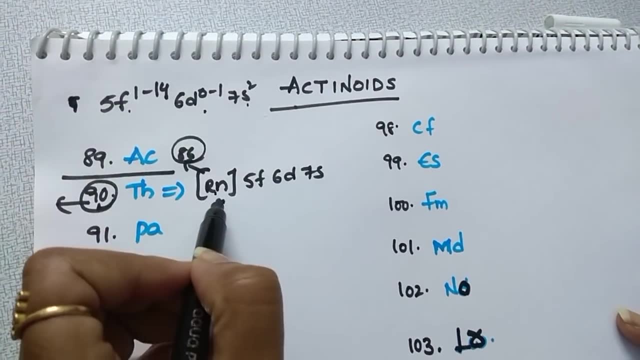 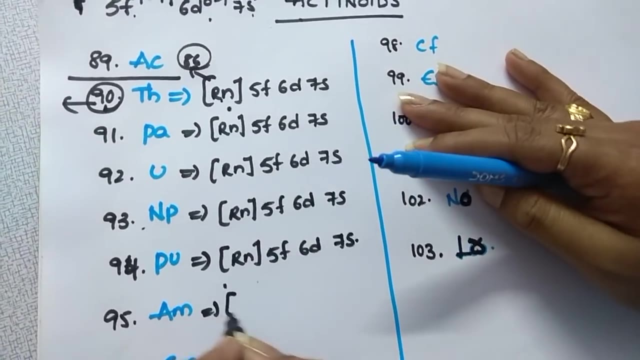 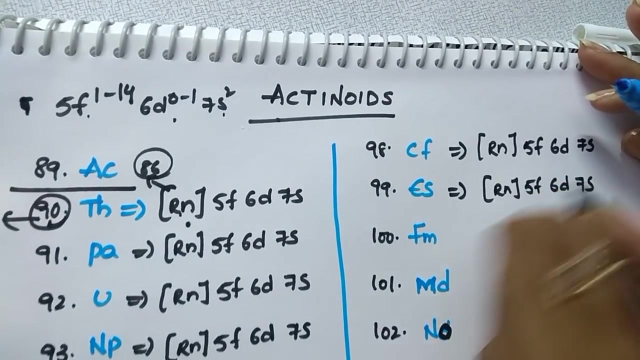 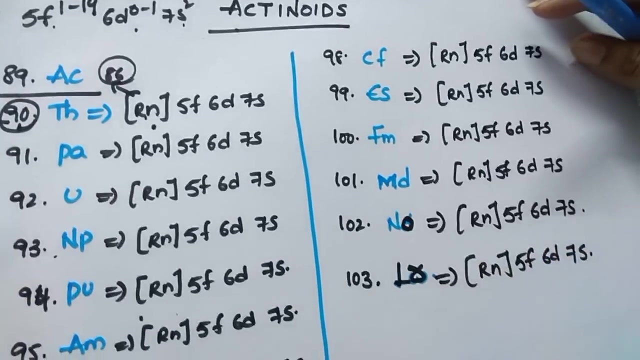 1 is just write down Radon 5F, 6D, 7S. Why we are taking Radon, students? Because near to the 90 atomic number the nearest noble gas is Radon. Some many know Radon 5F, 6D, 71, but we should write down Radon. 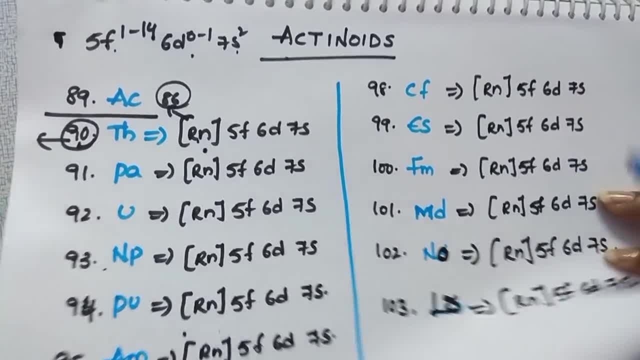 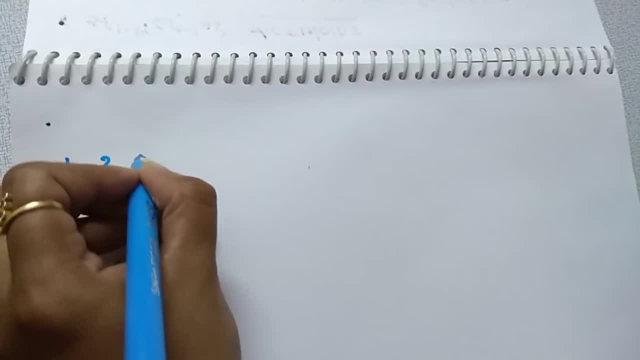 Radon 5F6D 7S. I write for all the elements. Now the trick is just write down the elements from numbers from 1 to 14,: 2, 3, 4, 5, 6, 7, 8, 9, 10. 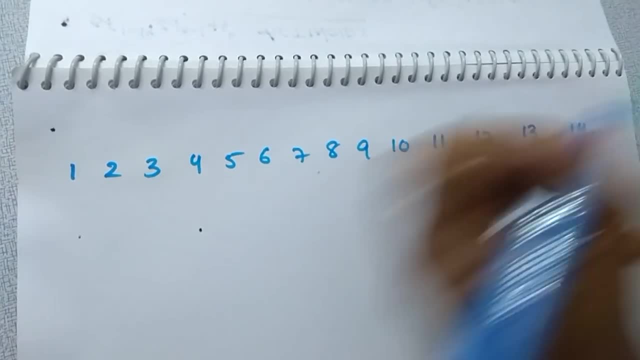 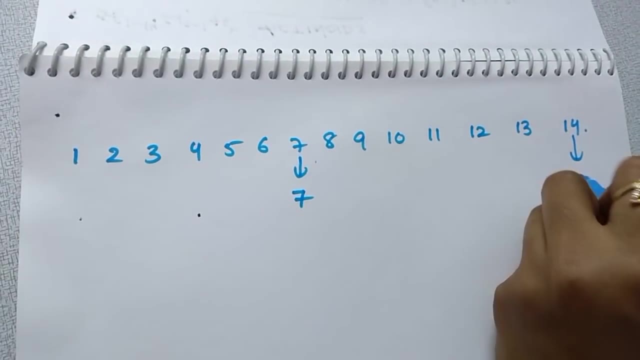 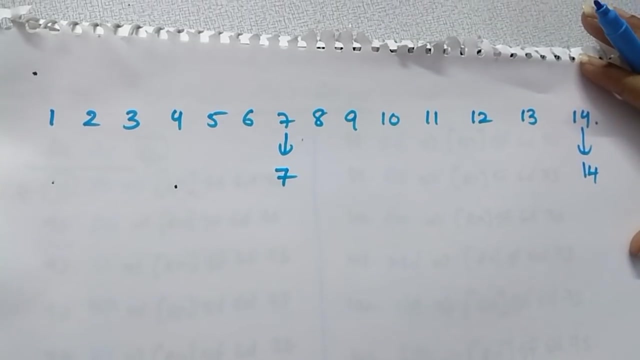 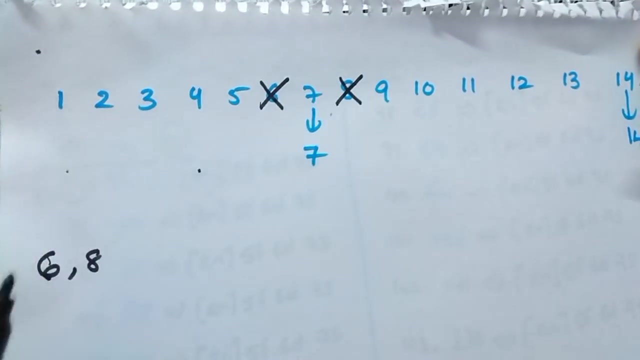 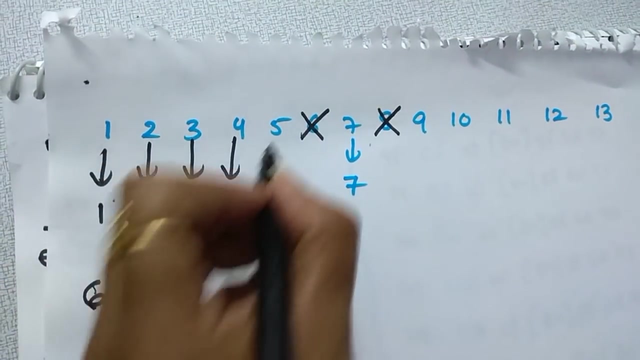 11, 12, 13, 14. For F, half filled, 7, which is more stable, and completely filled is more stable, that is, 14. no change in these two numbers and don't take the numbers 6 and 8. so 1, 2, 3, 4, 5. next number is 7 because 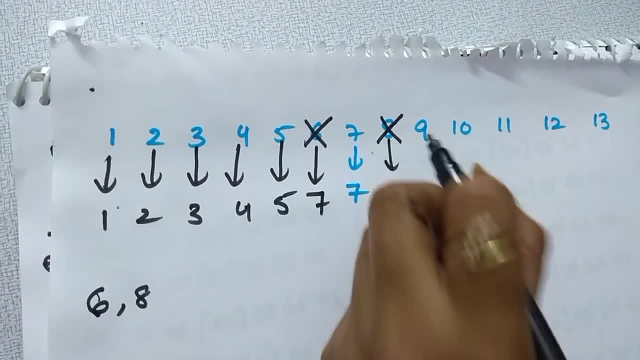 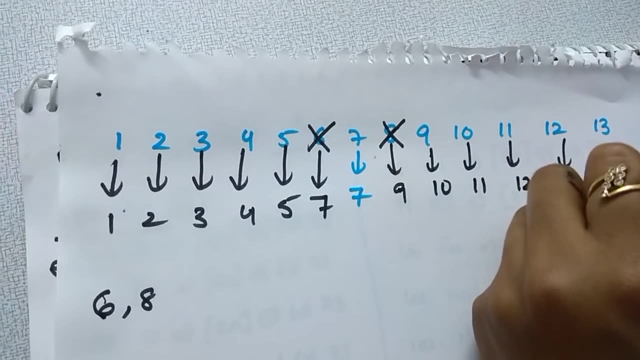 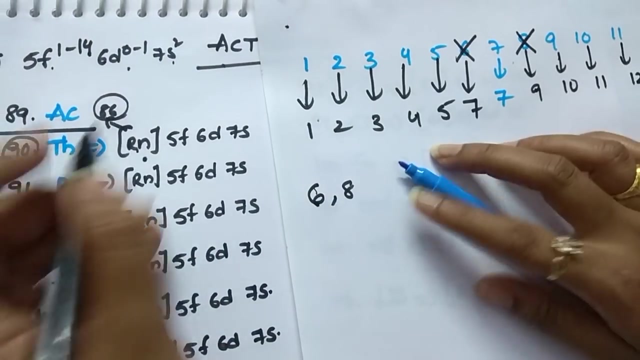 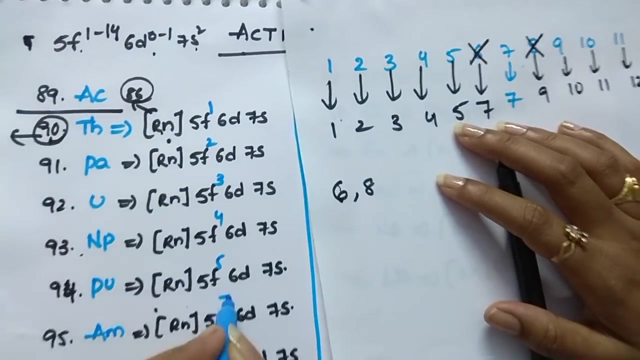 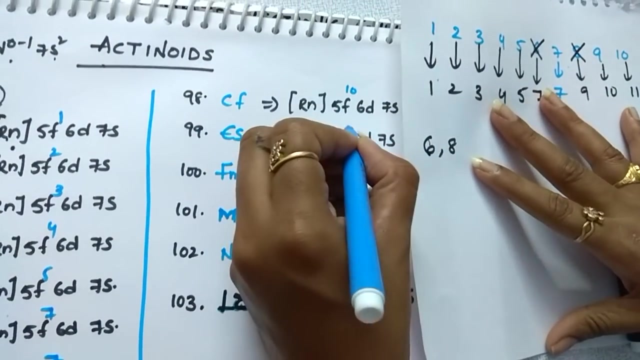 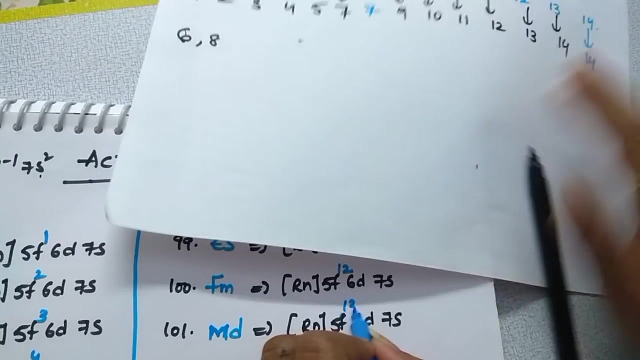 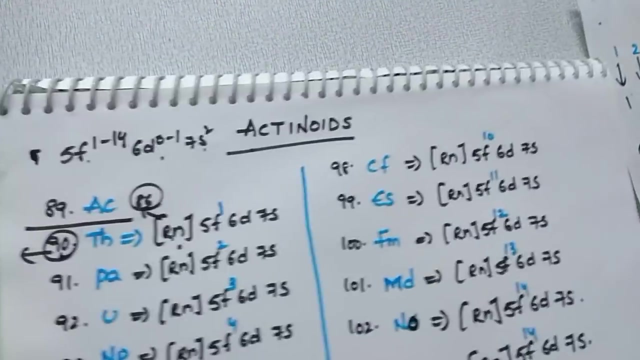 no 6, 8, not there- 9, 10, next 11, next 12, 13, 14. just fill these electrons in: F: 1, 2, 3, 4, 5, 7, 7, 9, 10, 11, 12, 13, 14, 14. we discussed that. s consists of two electrons, no change in. 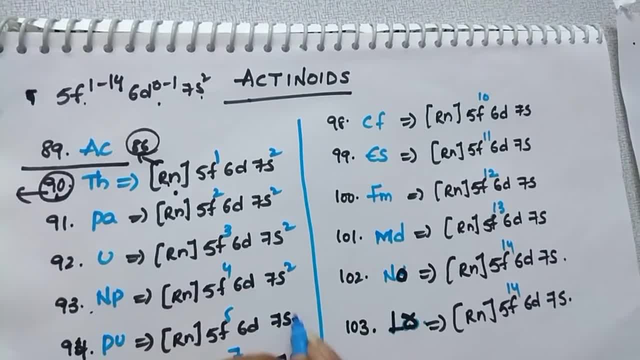 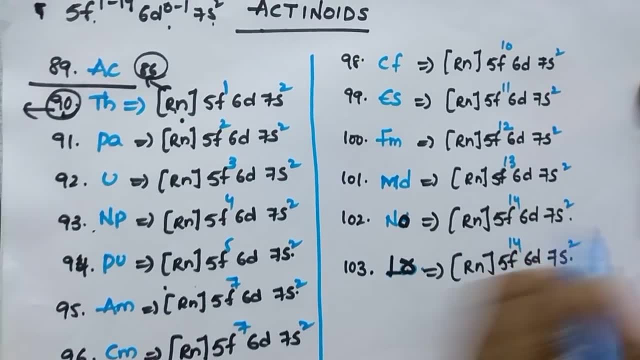 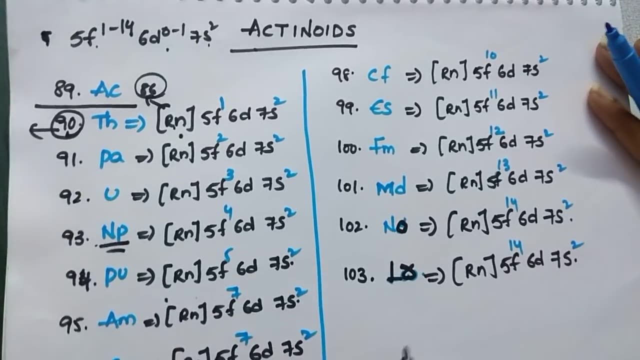 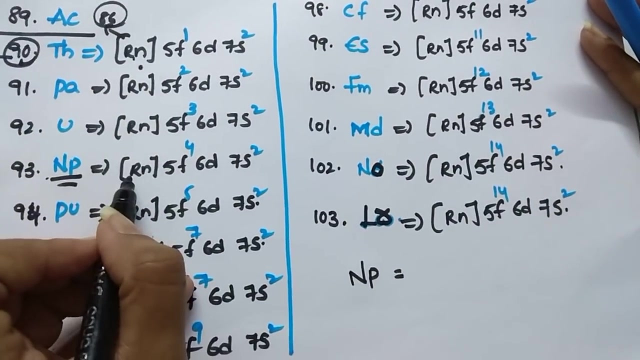 this. so fill two electrons in all the s orbitals. after filling this, what you have to do is suppose take out neptunium, neptunium electronic configuration. you want to write neptunium you already filled. radon means radon. atomic number is 86 plus 86 electrons. it has F, consists of four. 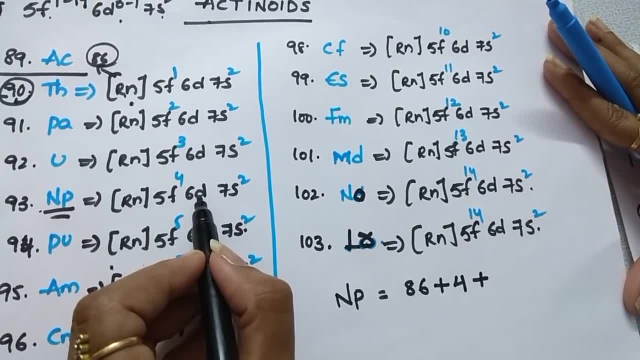 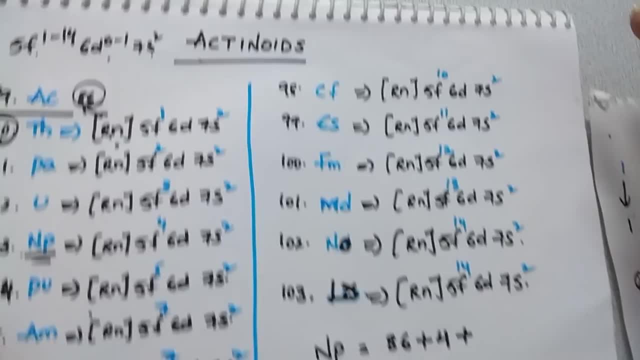 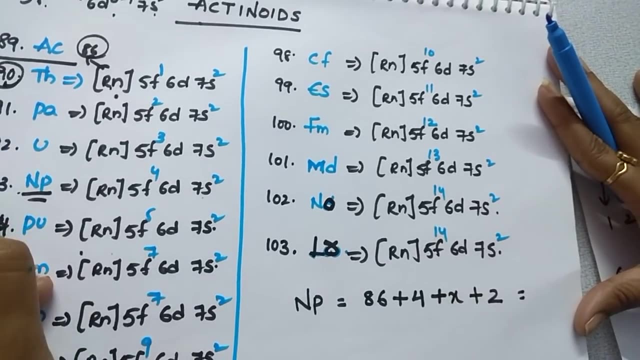 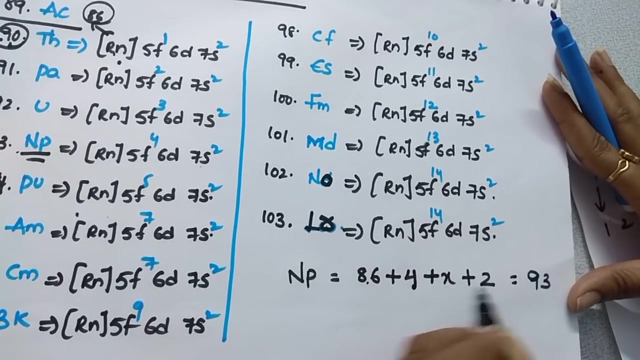 electrons plus 4 plus D, how many electrons it may has zero electron or it may have one electron generally creates a confusion to the students whether 0 or 1. so consider it as X plus s is having 2, the total sum should be equal to its atomic number of neptunium, that is 93, then 86 plus 4, 90, 90 plus 2. 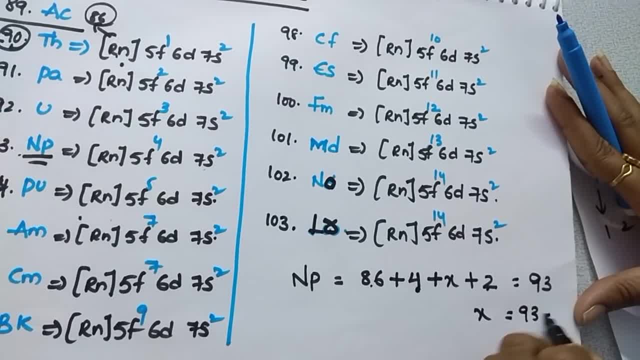 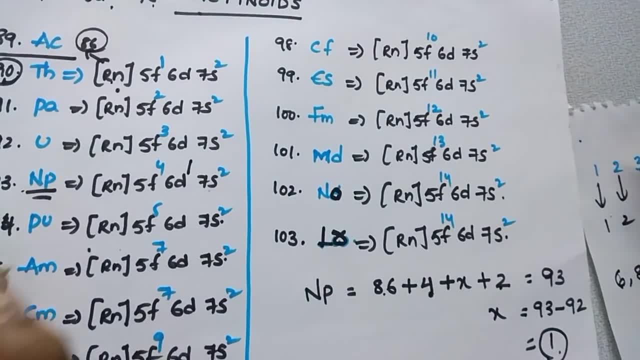 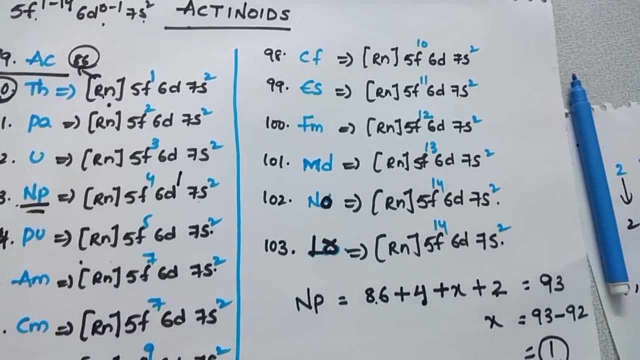 92, then X is equal to 93. if this 92 come this side, minus 92, then X is equal to 1. so the number of electrons in the D is 1. what is the configuration of neptunium students 5F4,, 61 and 7S2.. Let us find the electronic configuration for formium Formium. 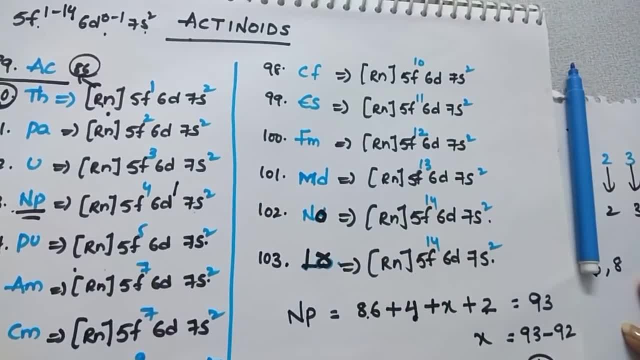 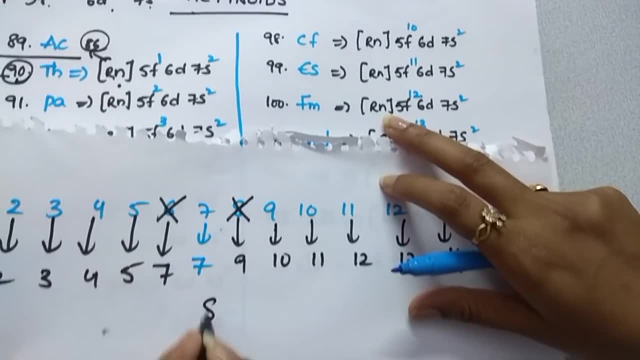 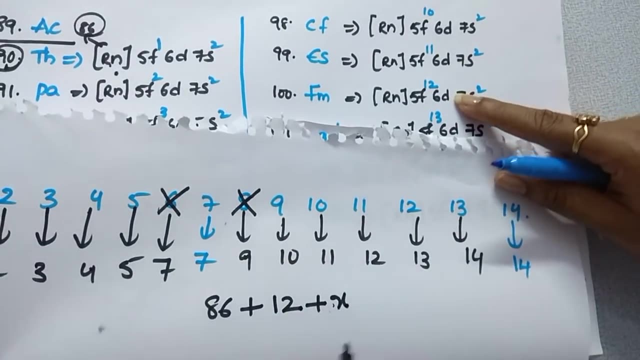 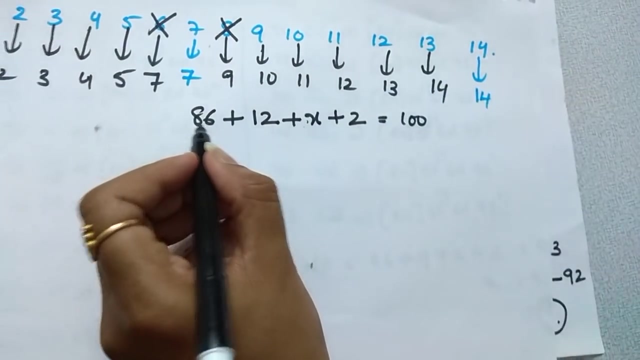 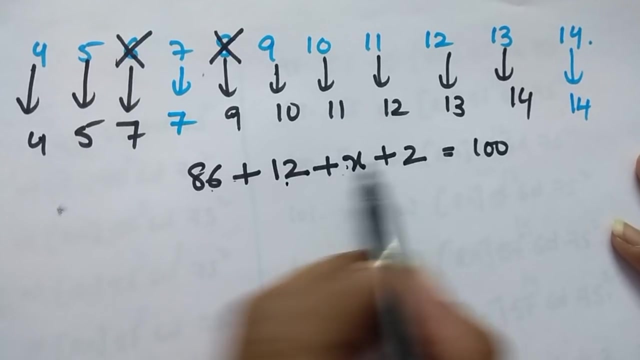 atomic number is 100.. We already filled radon. 86 plus F consists of 12 electrons plus D. how many electrons, we don't know. consider it as X plus S has 2 electrons, The total sum is equal to 100. Then add this: 86 plus 12,, 86 plus 12, 98,, 98 plus 200.. So X plus 100 is equal to 100. then 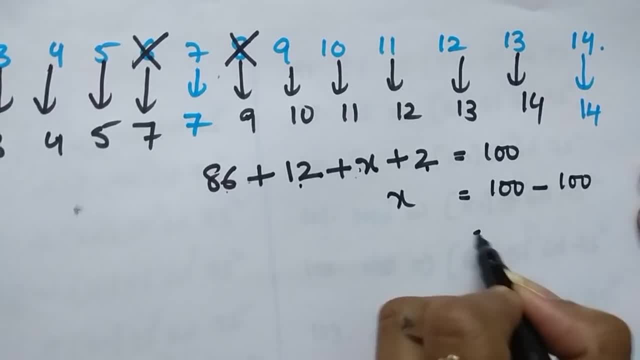 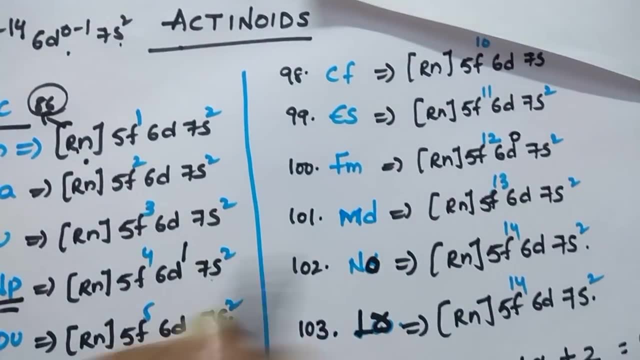 X is equal to 100 minus 100, 0.. The number of electrons in this D orbital is for formium is 0.. So what is the electronic configuration of formium? Radon, 5F14,, 6D0,, 7S2.. 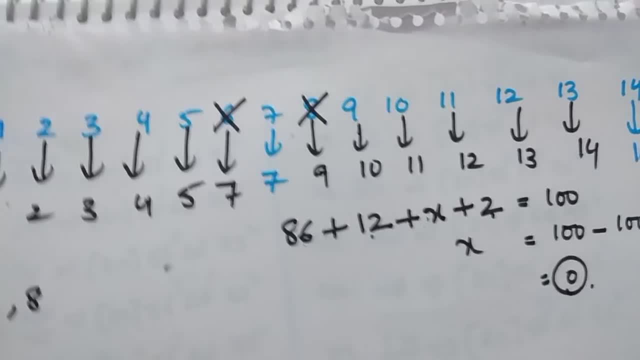 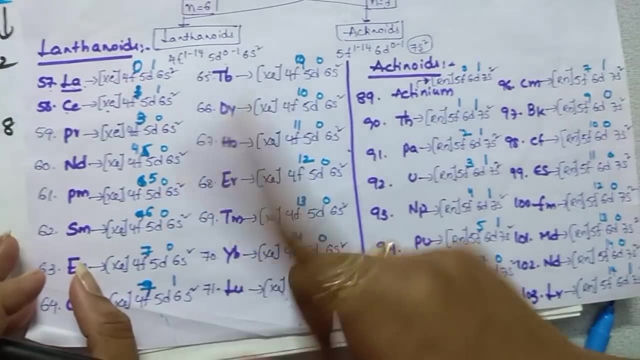 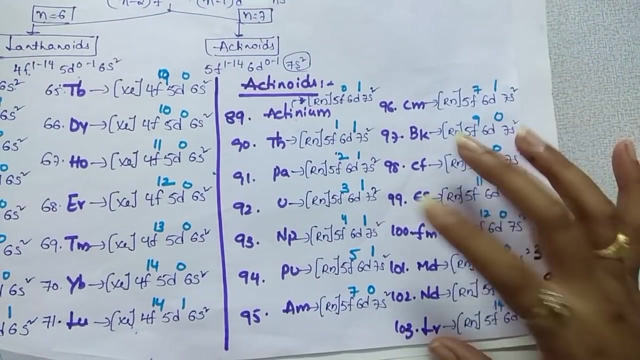 Just find like this for all the elements. then you get the configuration of elements like this. This is for lanthanides. in previous video I covered this once. go through the video. After getting the electronic configuration, what we have to do is just suppose you want to. 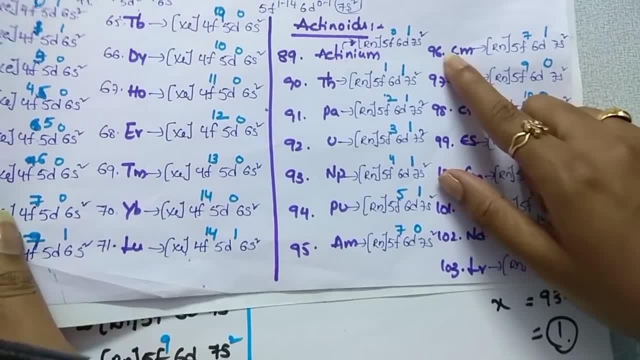 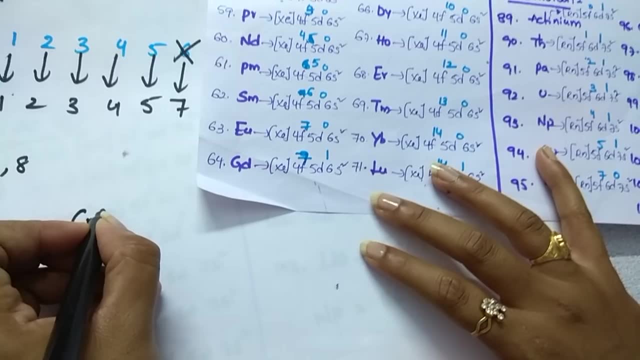 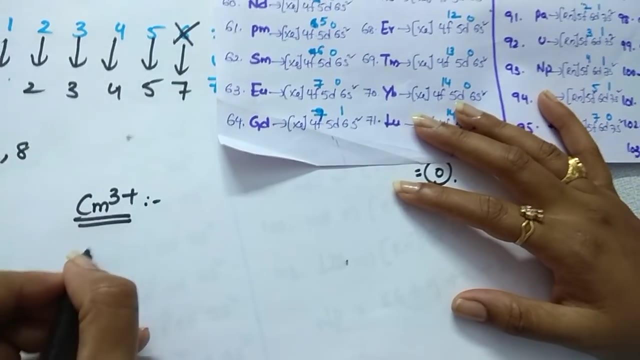 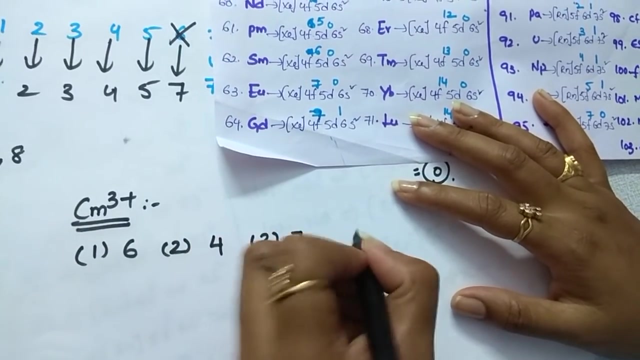 find the number of unpaid electrons. Curium the number of unpaid electrons. in the exam they asked CM3 plus: find the number of unpaid electrons. The number of unpaid electrons in CM3 plus: First option is 6,. second option 4,. third option 7, fourth option is 5.. The number of unpaid electrons: 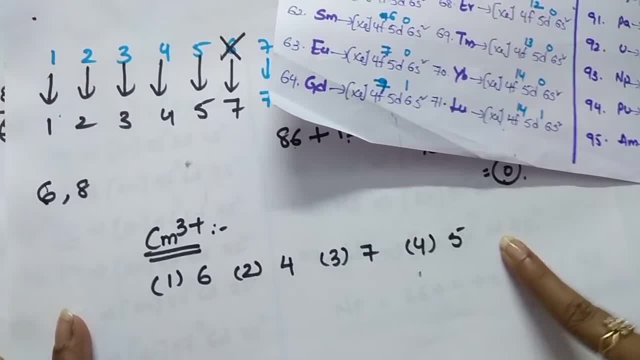 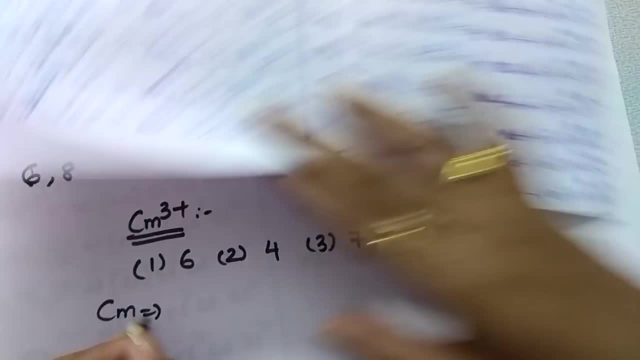 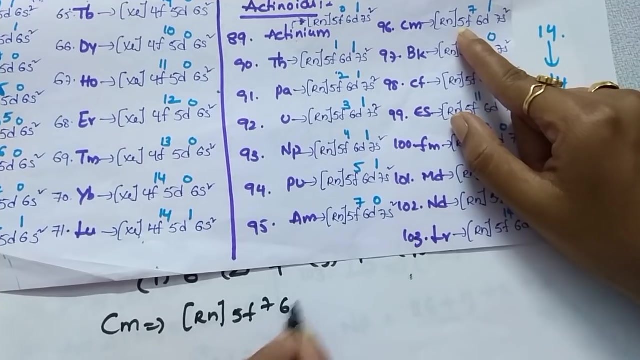 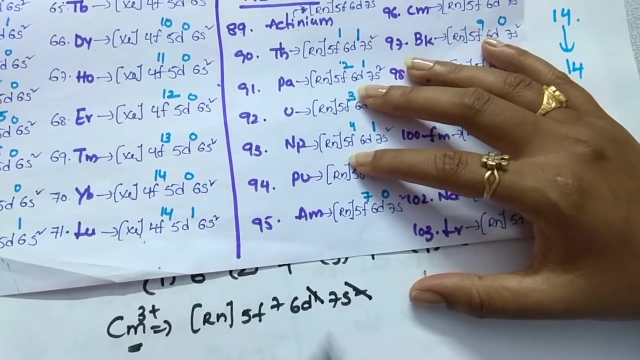 in CM3 plus is 6,, 4,, 7,, 5.. Then if you know the electronic configuration, only you can attempt this question. Then write the CM electronic configuration. What is the electronic configuration? Radon 5F7,, 6D1,, 7S2.. In plus 3 state: remove 3 electrons, 2 from S, 1 from D, So D becomes 0, S also. 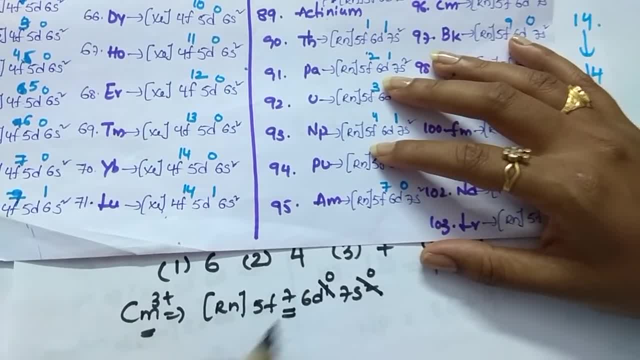 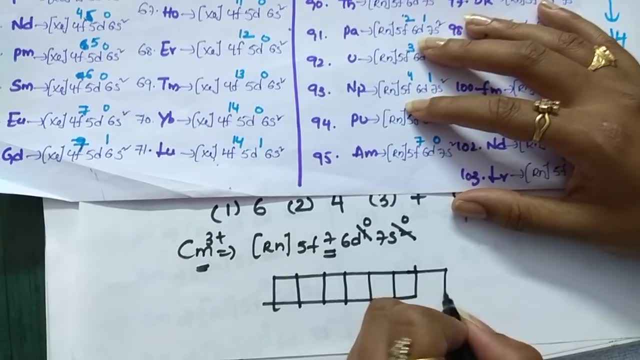 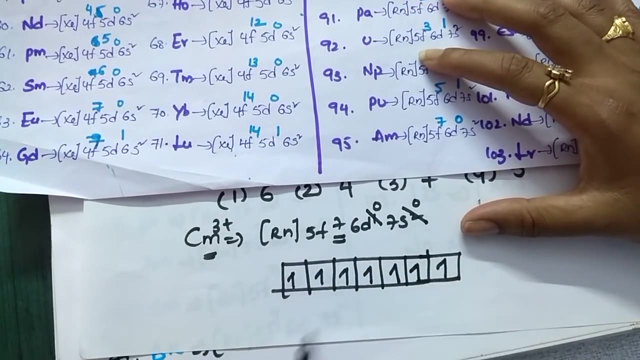 has 0, no electrons. F has 7 electrons: 3,, 4,, 5,, 6, 7.. 7 orbitals: 1,, 2,, 3,, 4,, 5,, 6, 7.. So how many unpaid electrons are there? N is equal to 7.. So which? 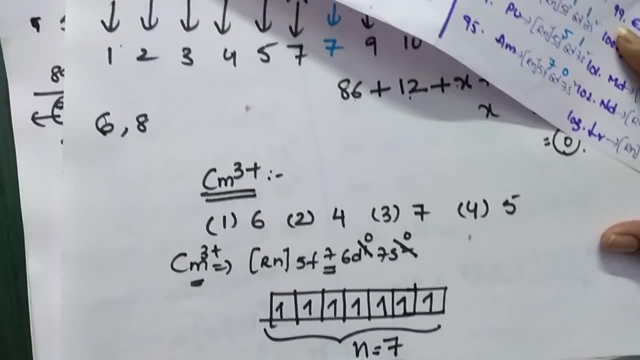 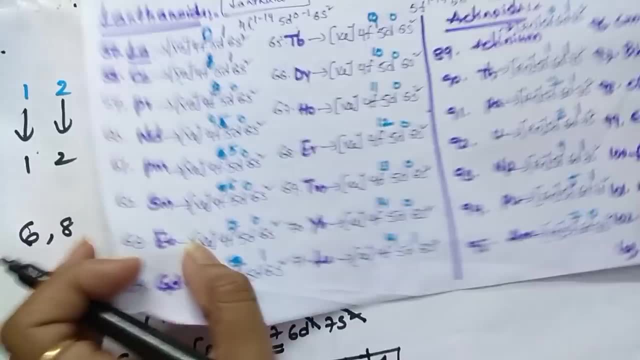 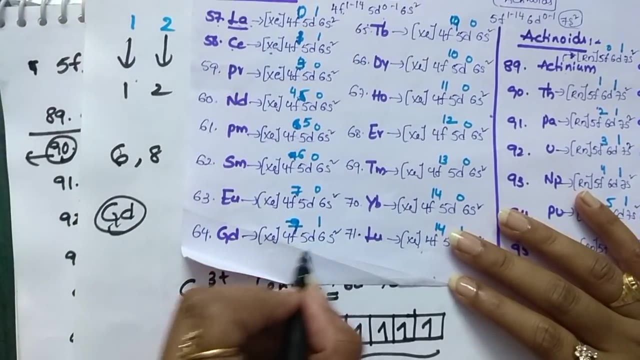 option is correct, students. Number of unpaid electrons is 7.. So which option is correct? Third option: Let us find the number of unpaid electrons for D block element like gadolinium. Gadolinium, Most important thing is gadolinium. they asked the. 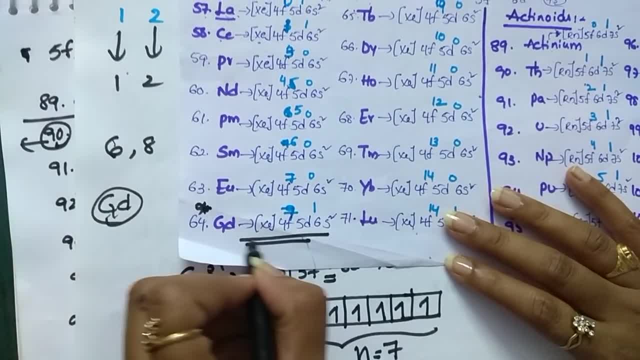 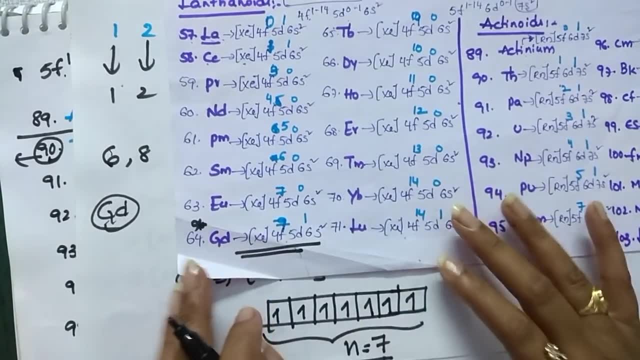 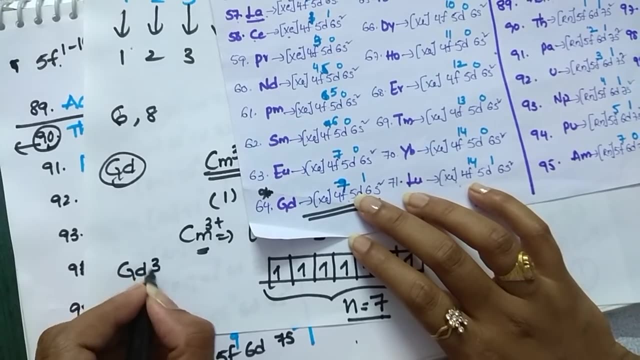 electronic configuration. What is the electronic configuration? Xenon 4F7,, 5D1, 6S2.. I covered about this lanthanides in previous video. Once, go through that. and what is the? what are the number of electrons present in GD3 plus How many number of unpaid electrons? remove In plus 3, state you. 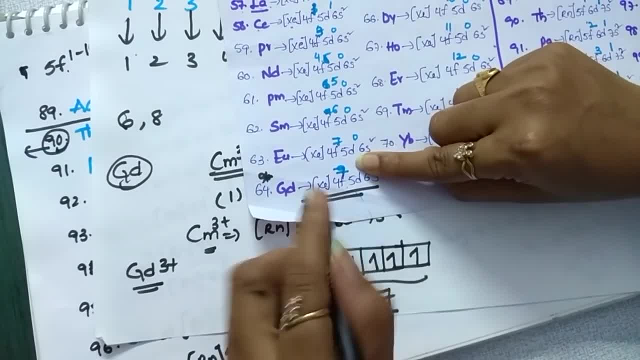 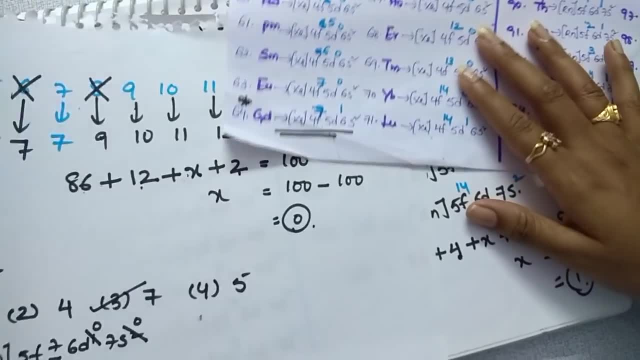 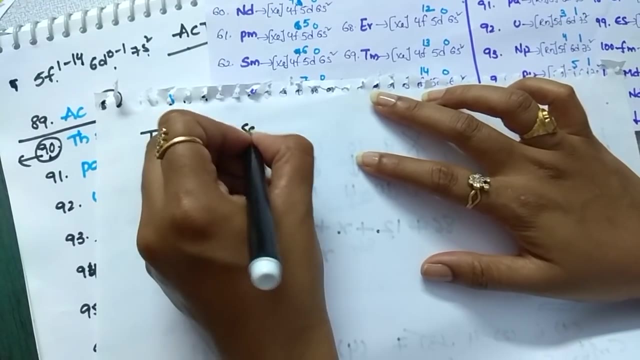 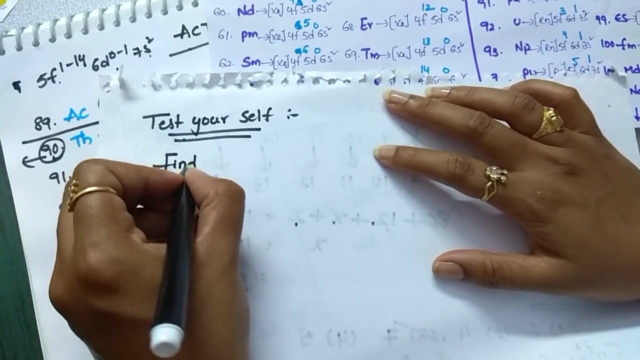 have to remove 3 electrons, 2 from S, 1 from D, Then 7, 7. just fill in the F, we get number of unpaid electrons is 7.. And one more question is: test yourself. question: Find the number of unpaid electrons. 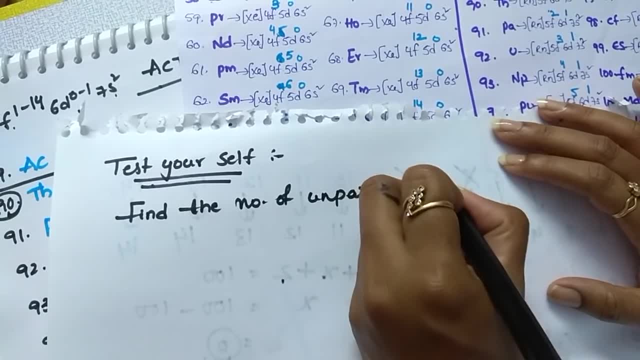 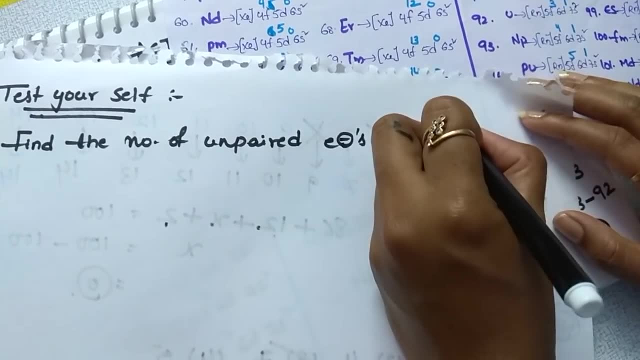 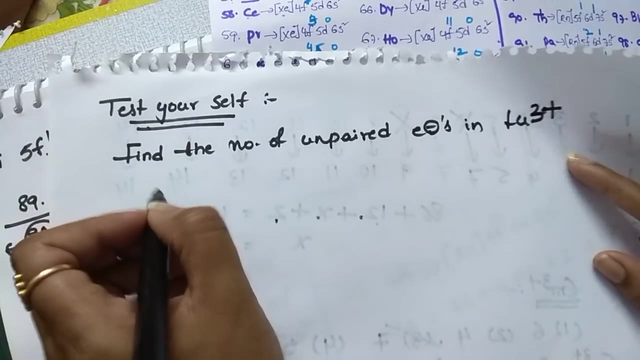 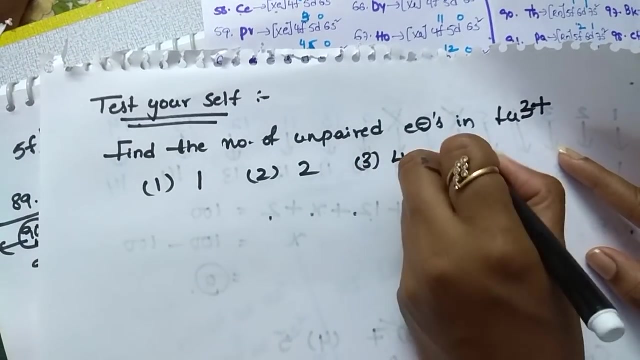 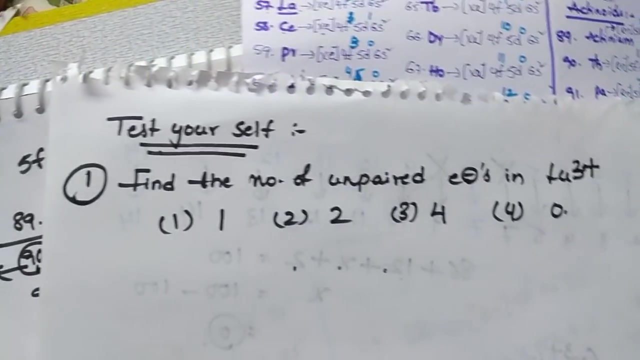 electrons in LU2 plus, LU3 plus. Find for LU3 plus Option 1, 1.. Option 2, 2.. Option 3, 4.. Option 4, 0.. This is question number 1.. By using this trick, find the number of unpaid electrons And, coming to this, by using this electronic configuration, you can find the magnetic property. 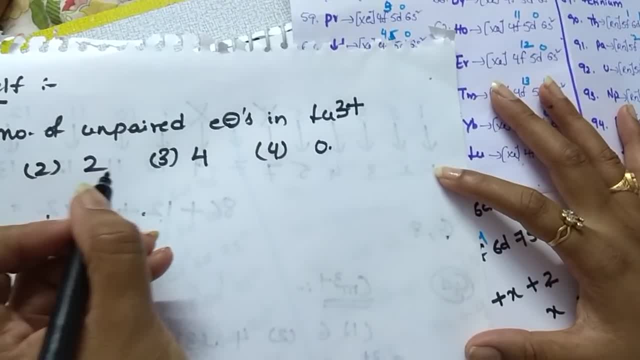 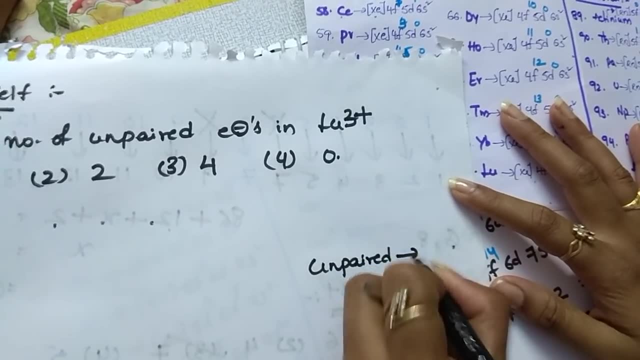 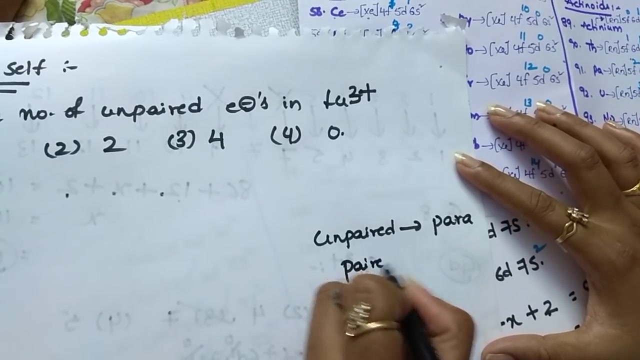 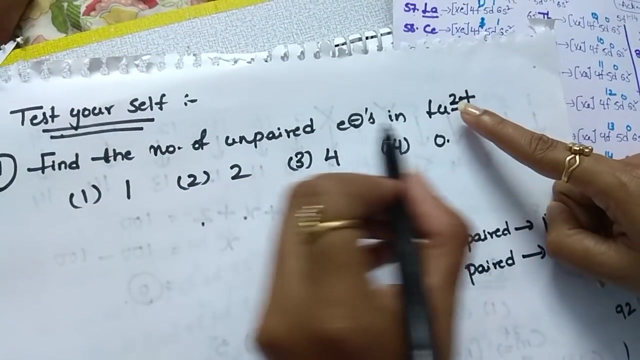 Suppose, after finding the number of unpaid electrons, if the iron is having the unpaid electrons, unpaid electrons, then the particular iron is para magnetic in nature. If it is not having unpaid electrons, all are paid, then it is dia magnetic. Then, after finding the number of unpaid electrons, 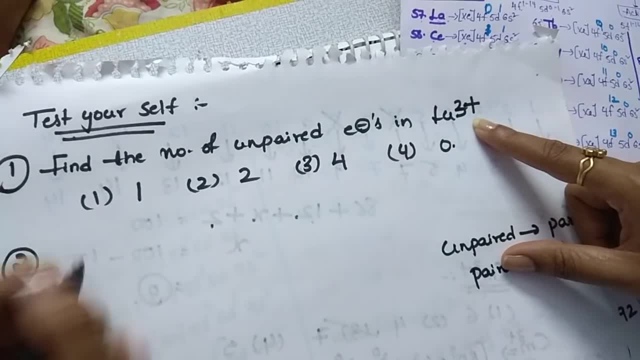 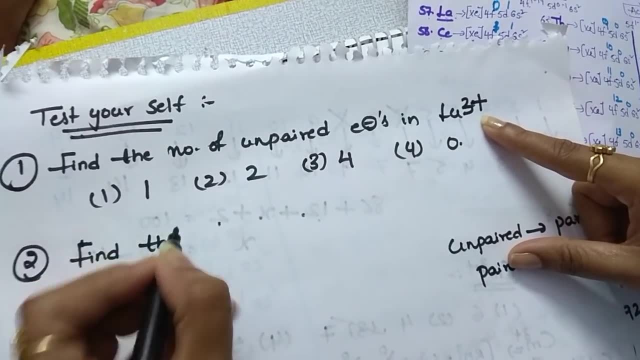 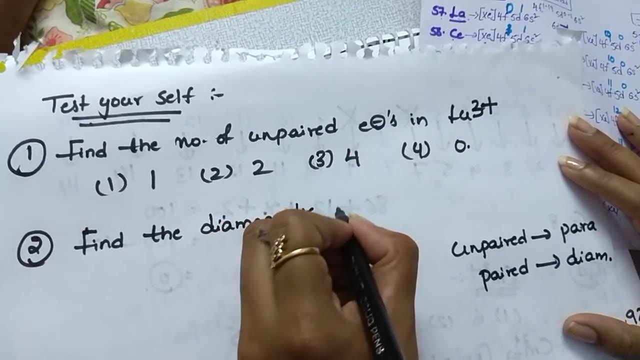 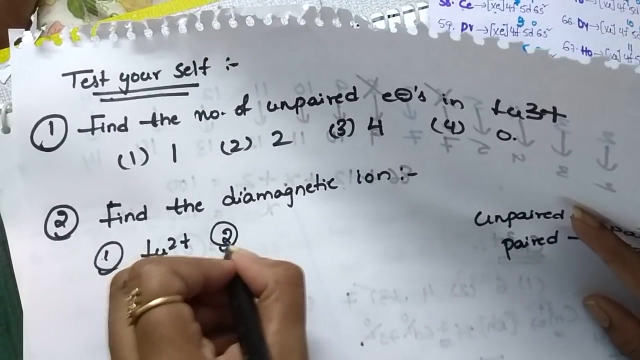 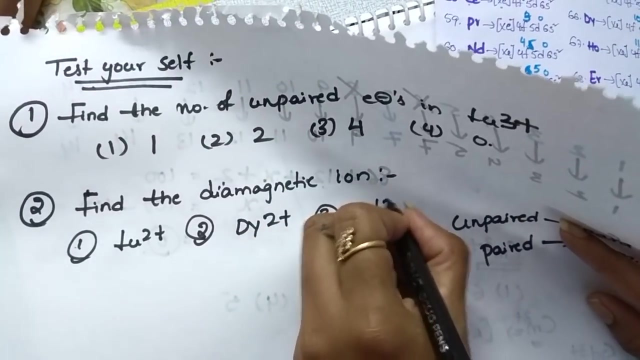 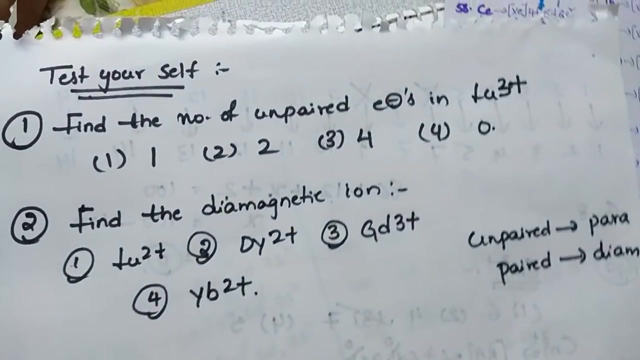 in Lu3+. what you have to do is question number 2, find whether it is para or dia. find the diamagnetic- suppose diamagnetic- ion from the following: first one is Lu2+. second option is Dy2+. third option is Gd3+. fourth one is Yb2+. By using this trick, what you have to do 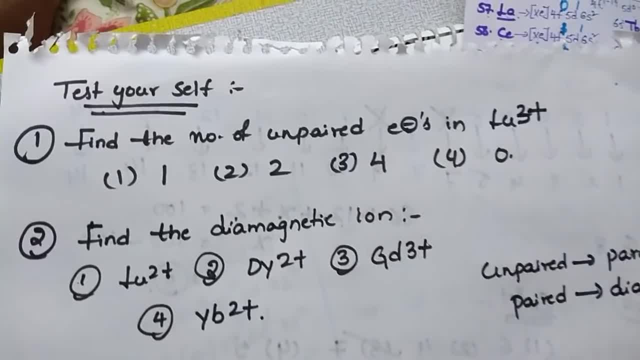 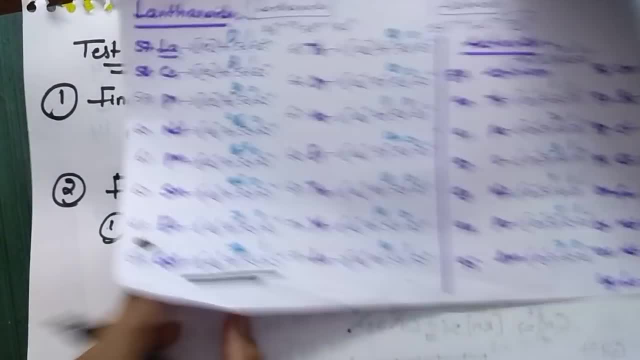 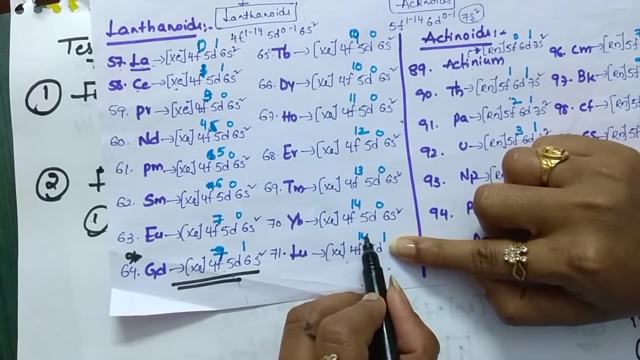 students, you have to find the diamagnetic ion. how to find the diamagnetic ion? if suppose Lu2+? I will tell you: Lu2+ is lutetium. lutetium in 2 plus state removed two electrons. if you remove two electrons, F is completely filled, no unpaired electrons, but D is having 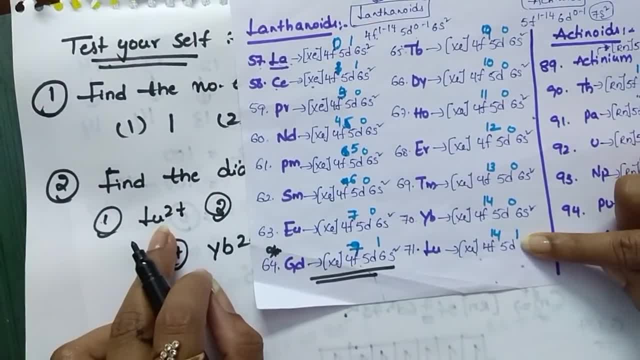 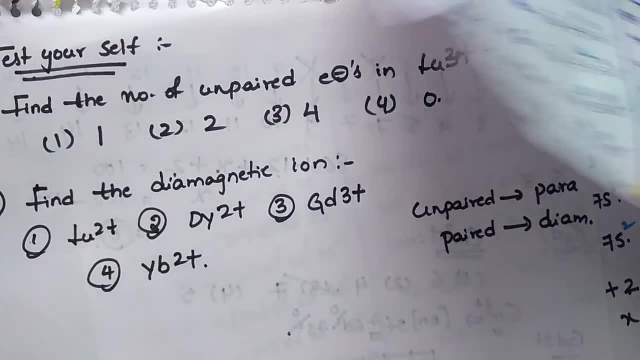 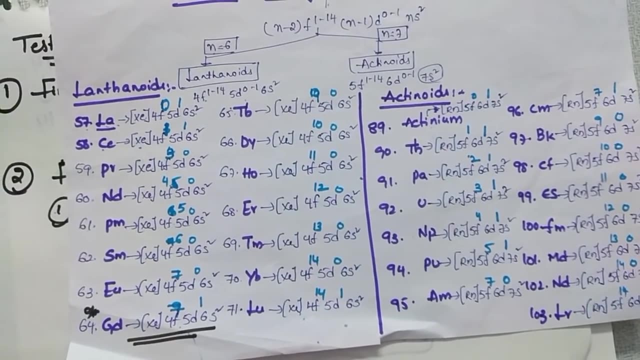 one unpaired electron. so Lu2+ is having one unpaired electron. if unpaired electron is there, it is para. so this option is not correct like that. find out which is having completely filled by using the electronic configuration. after finding the magnetic moment, I will tell you. 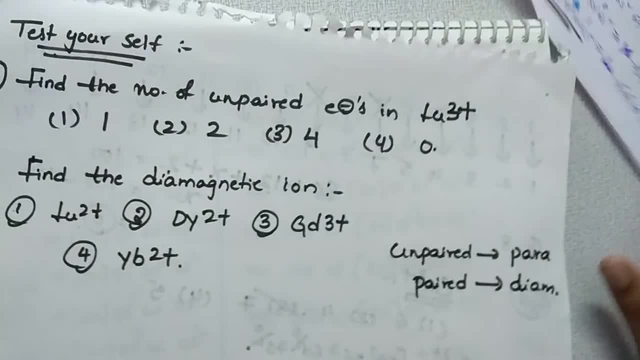 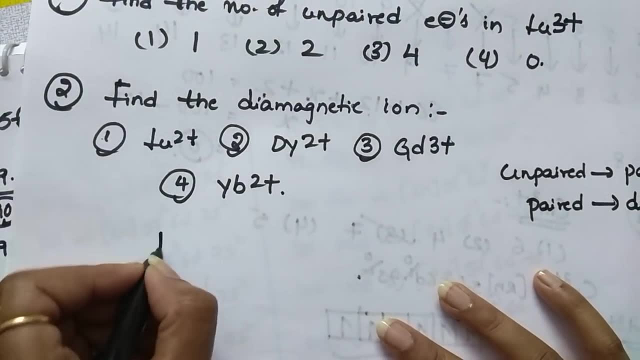 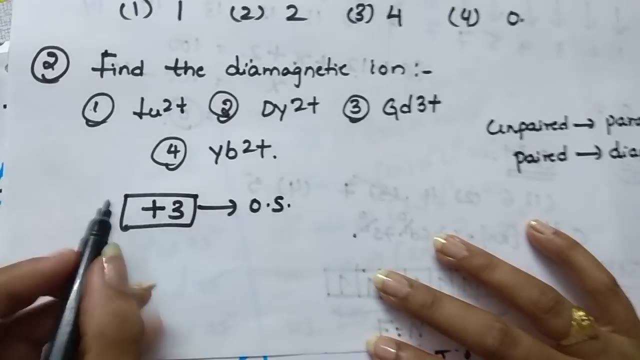 one more trick also. you can find the oxidation state which is more stable. the common oxidation states for lanthanides and actinides is plus 3, plus 3 is the common oxidation state. suppose if we discuss about the lanthanides, they shows not only plus 3, they shows plus 2 and 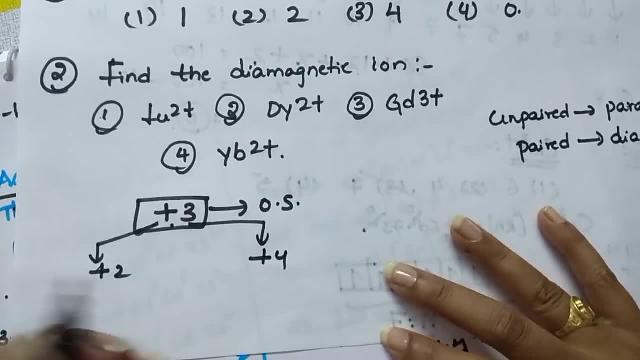 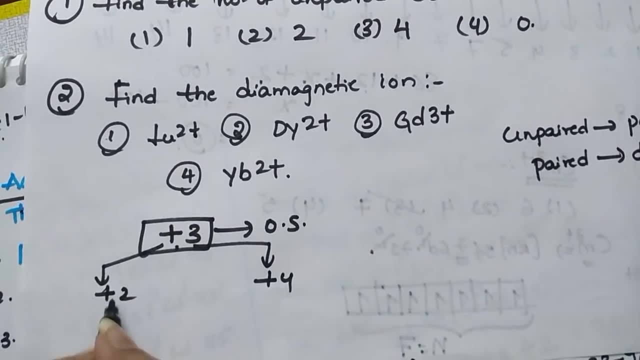 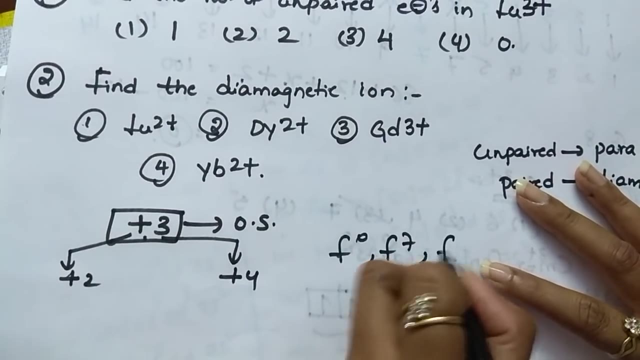 plus 4 also ok, but the common stable configuration is plus 3,. in some cases they show plus 2 and plus 4,. actually, when they show plus 2 and plus 4 is either they have no electrons in F or half filled 7 or completely filled 14,. to get the stability right, and even though 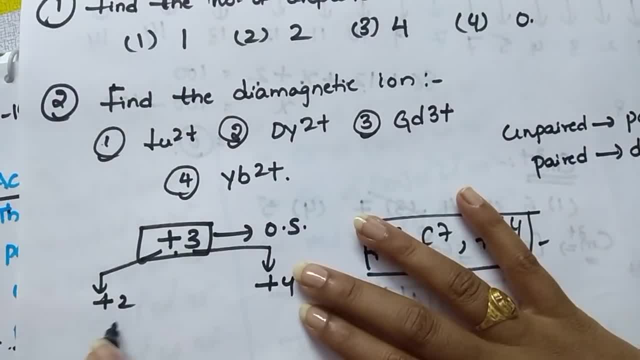 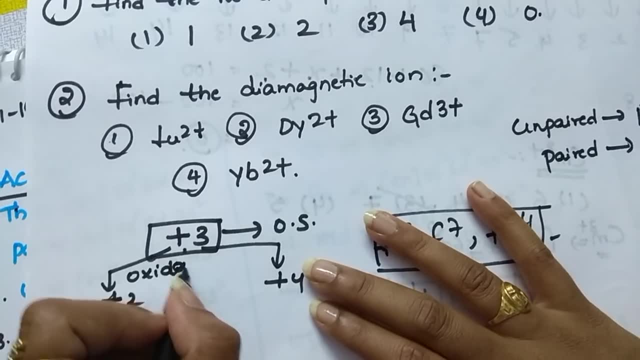 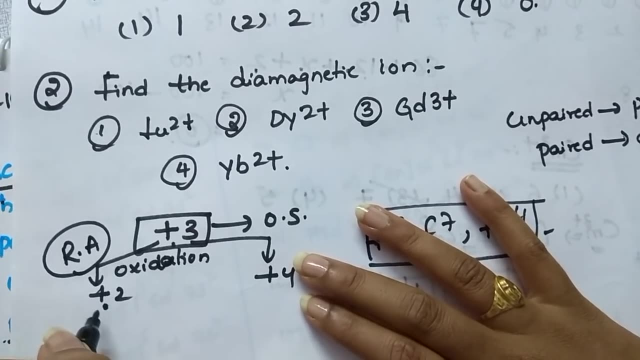 plus 3 is a more stable oxidation state. if in plus 2 it is there, it try to oxidize into plus 3, if it is undergoing oxidation itself, it is undergoing oxidation. it acts as a reducing agent. the ion which is there in the plus 2 state it tries to convert into plus 3, in this case. 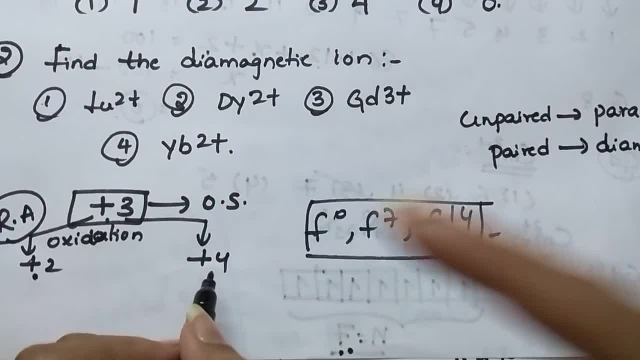 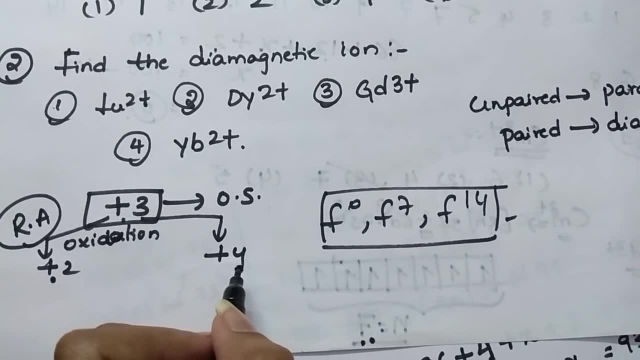 it acts as an reducing agent and suppose, if it is there in the plus 4 state in these 3 forms, either in F0 or F7 and 14, it tries to convert into F3, plus 3 state, plus 4 it. 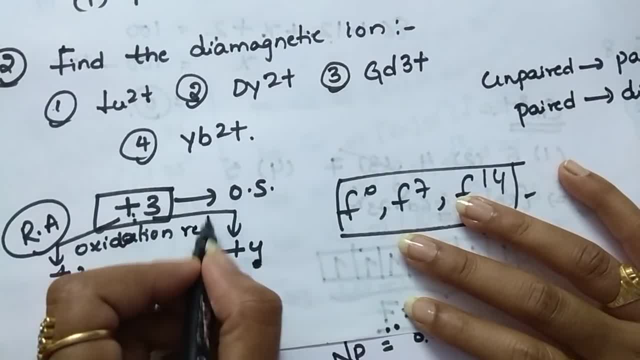 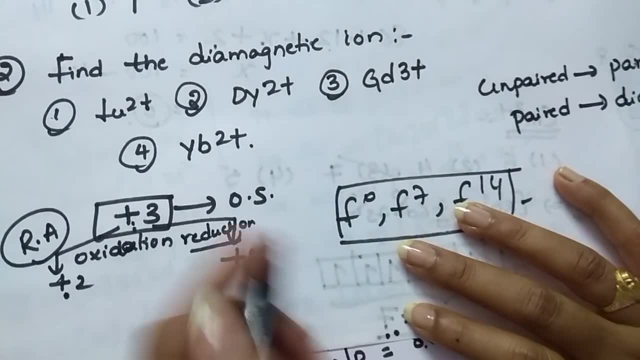 tries to convert into plus 3, means it undergoes the reduction. during this process, an ion is itself undergoing reduction and it makes other element to undergoes oxidation, so it acts as an oxidizing agent. Let us see an example. Let us see an example. 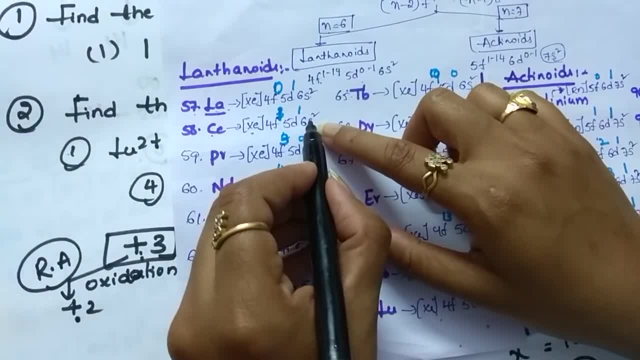 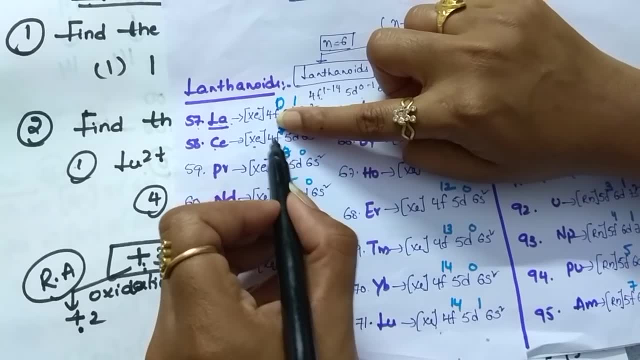 Serium, Serium. if it lose 4 electrons, 2 from S, 1 from D and 1 from F, total 4 electrons. if it lose, it has 4F0 configuration, means no electrons in the F, even though it is present. 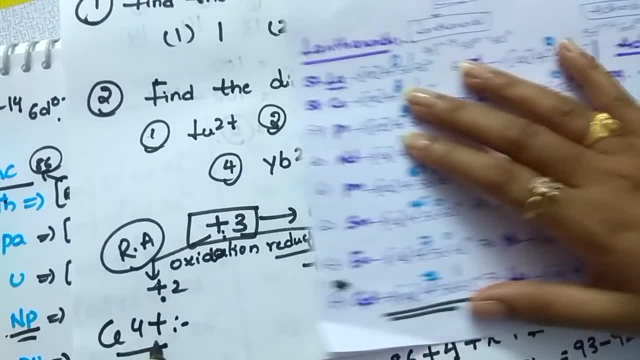 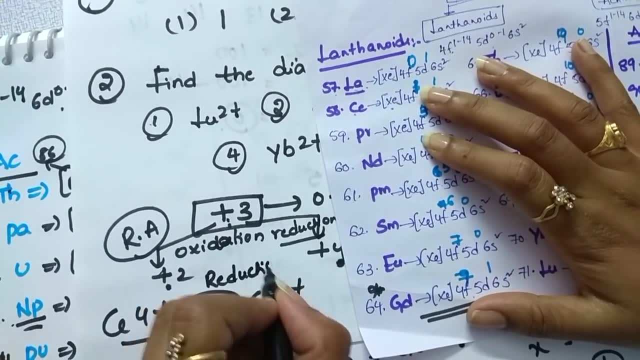 in Serium plus 4 state. plus 3 is the most stable, so it try to convert into plus 3, during this time means it is undergoing reduction, reduction gain. it gain an electron and it undergoes the reduction and during this process, 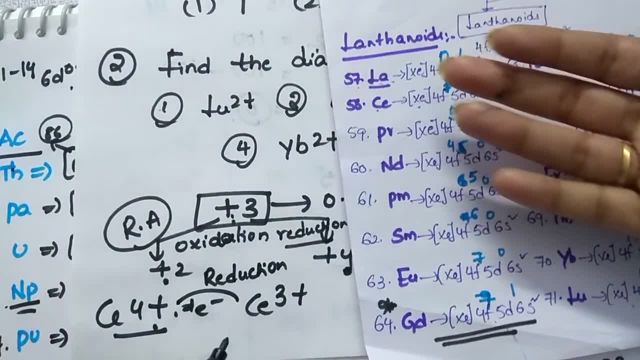 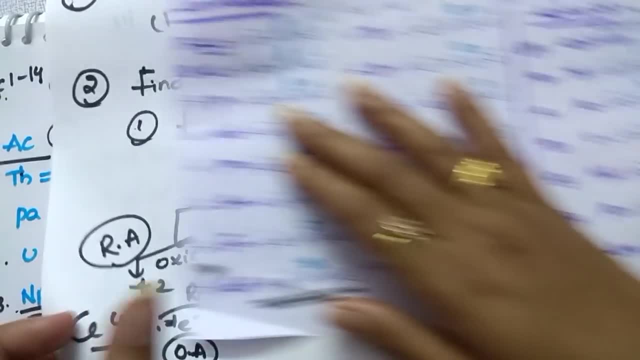 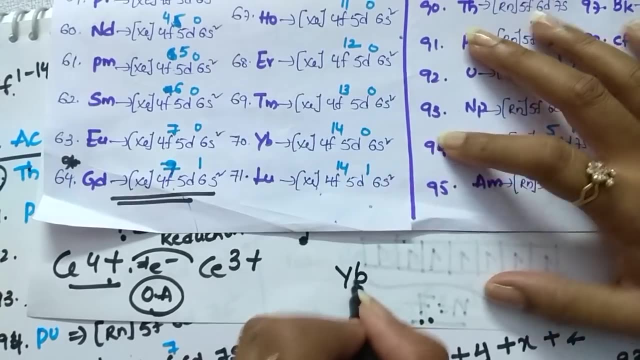 It is itself undergoing reduction and makes the other element to undergo oxidation, so it acts as an oxidizing agent. Serium plus 4 is an good oxidizing agent. and suppose, if you see Lutetium or Ytterbium, Ytterbium, Ytterbium, which is in plus 2, state in plus. 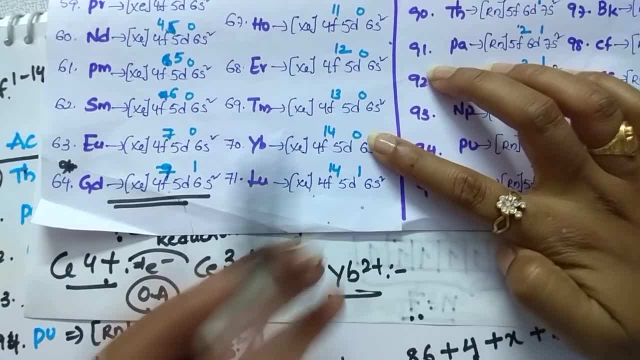 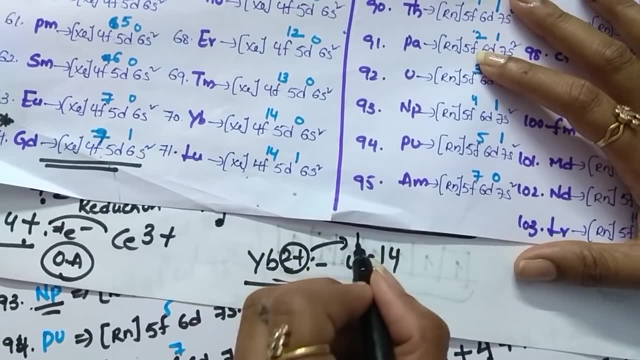 2, remove the 2 electrons from the S. so how many will be there? 4F14, right, stable, but even though it tries to convert into plus 3 state, Which is a common means, from plus 2 to plus 3, increase in oxidation number, we call it. 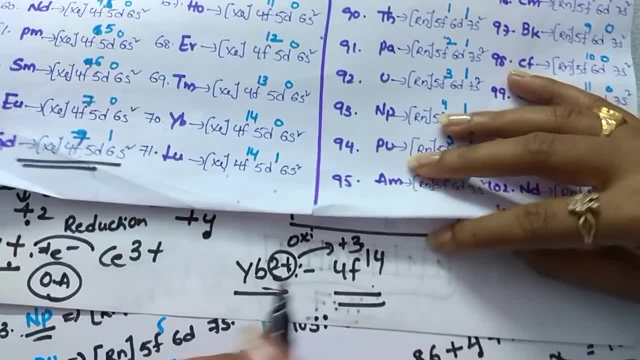 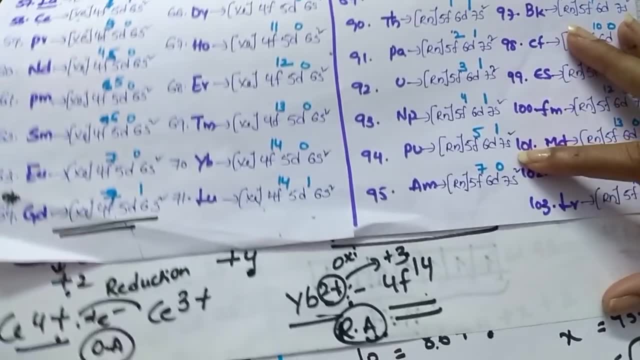 as oxidation right means itself undergoing oxidation and makes the other element to undergo reduction, so it acts as a reducing agent. it acts as a reducing agent. So by using this trick, you can find the electronic configuration. number of unpaired electrons. 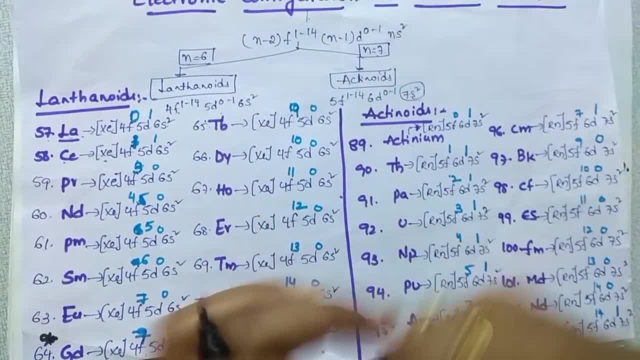 magnetic properties and oxidation state, which is the most stable state, and oxidizing and reducing agent. I hope you like this video. thanks for watching. 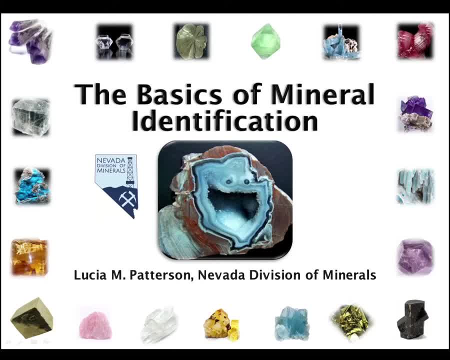 Hello, this is Lucia, a geologist with the Nevada Division of Minerals. I would like to welcome you to this video in which we will review the basics of mineral identification. In this video, we will discuss the tools we have to help us identify minerals and you will be introduced to many terms commonly used when identifying minerals. 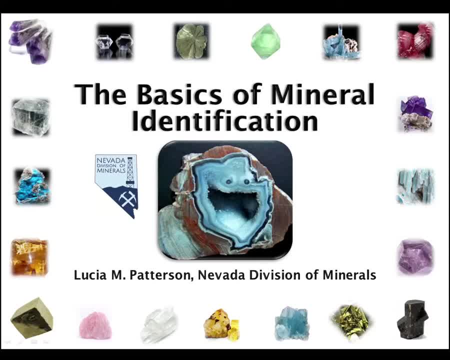 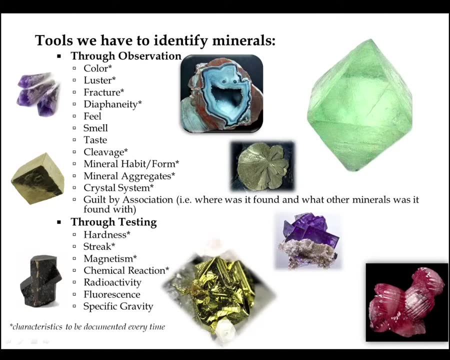 At the end of this video we will identify a couple minerals together and hopefully you will be ready to strike out on your own mineral identification adventure once we are done. Mineral identification is both challenging and fun. If it were simple, everyone would do it, But as with most anything that is challenging, the more you practice, the better you get. 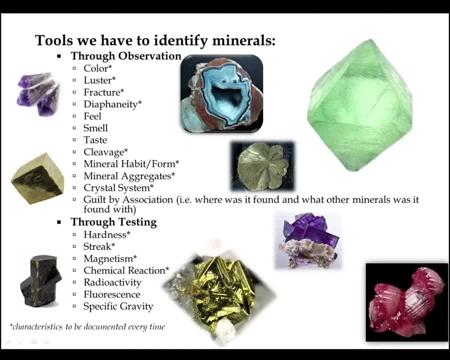 We have several tools that help us to identify minerals. Some are simple observation, like mineral color, luster, feel, smell or taste, and some, through actual tests, perform on the minerals, such as hardness, streak or condition. Mineral identification is a very important part of chemical reactivity. Not every observation or test needs to be performed every time. The tests and observations utilized most often are noted by asterisks on this screen. Let's review the tools. 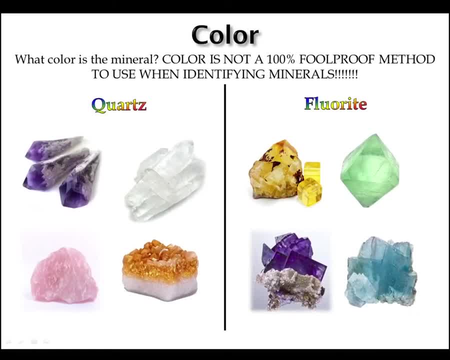 Color. Color is very important to note and most of the time it can lead you in the right direction for mineral identification. But color is not a 100% foolproof method. On the left we can see four different color varieties of quartz, And on the right we see four different color varieties of fluorite. 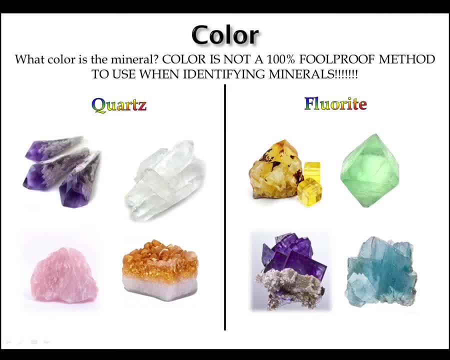 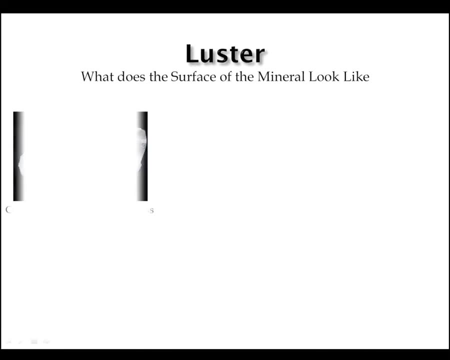 You should always document the color. However, if all other observations and tests point to another mineral except the color, don't disregard that mineral based on color alone. Luster- Luster of a mineral is commonly described as being glassy or viscous.